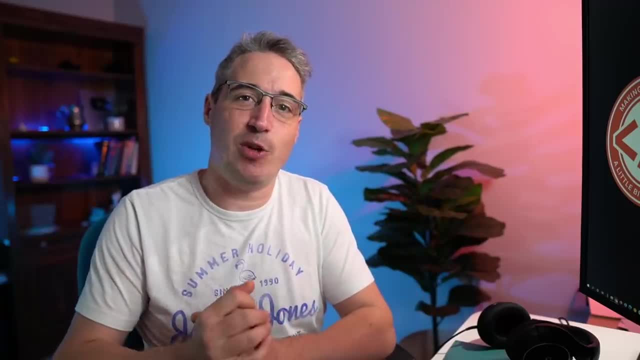 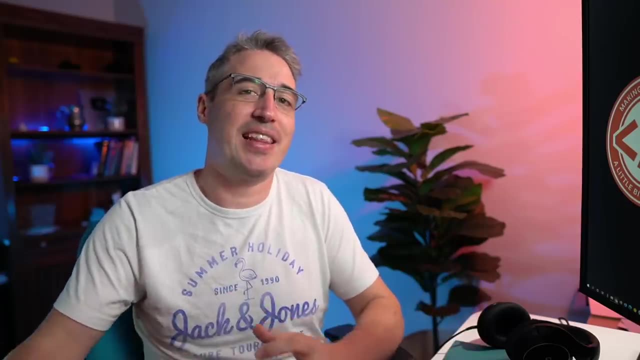 deeply in love with CSS And, if not in love with it, at least to be a little bit less frustrated by it. and I know responsiveness is something that I know people get very frustrated by, so I'm hoping I can help you take that frustration away with these five tips. Back when I first making websites, I didn't even have to worry. 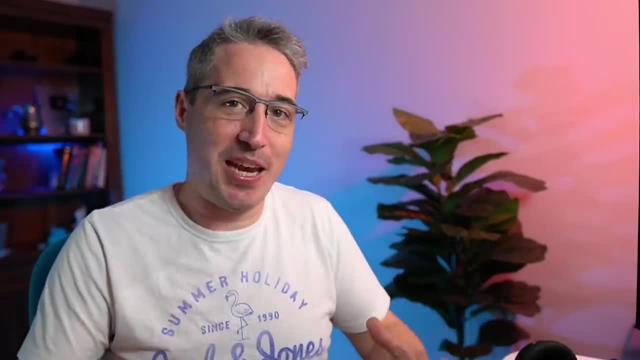 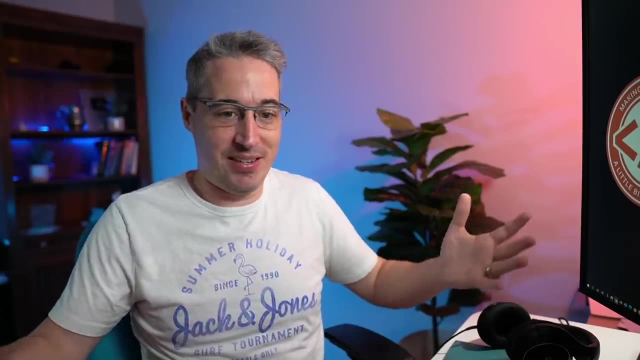 about making them responsive. We had a lot of other things that were a real pain, but we had a fixed size. you throw it in there, you get it working on that and we didn't have to worry about anything because we didn't have this whole range of insane devices and everything from giant monitors to 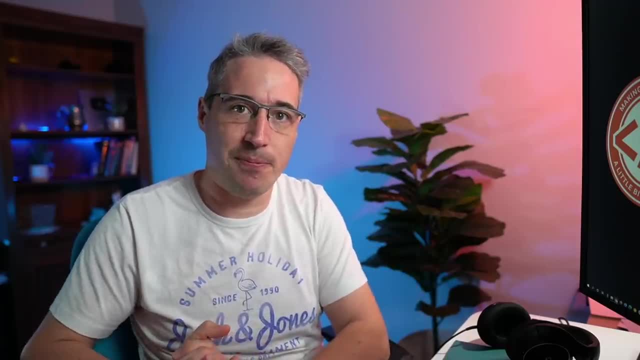 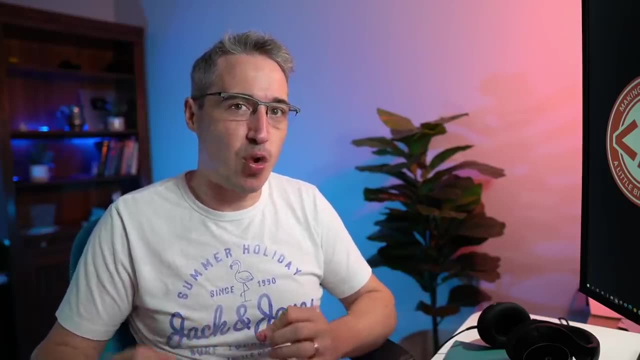 little tiny phones and even watches and everything In between. when responsiveness first started becoming a thing, we had a lot of obstacles in our way because we didn't necessarily have the tools to properly deal with it at the time. but we have a lot more now. but 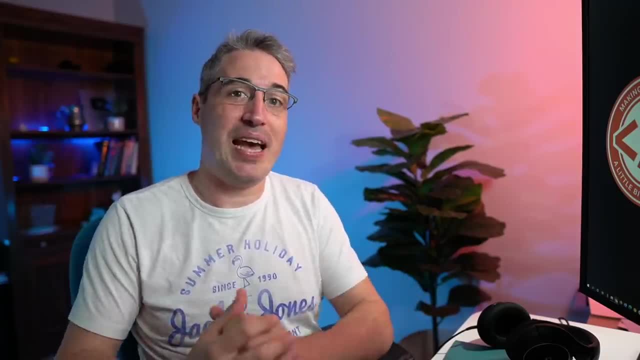 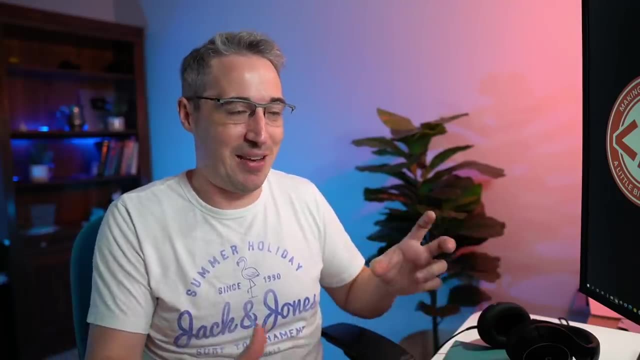 before we even get into any of those tools. my first tip revolves around having the right mindset, and this applied back when we were doing it back in the day, when things were just starting to change and we're getting away from having like two sites. we had to maintain your mwebsite, which was like the mobile version. 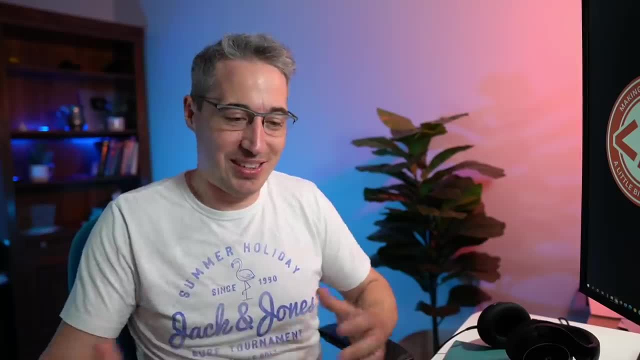 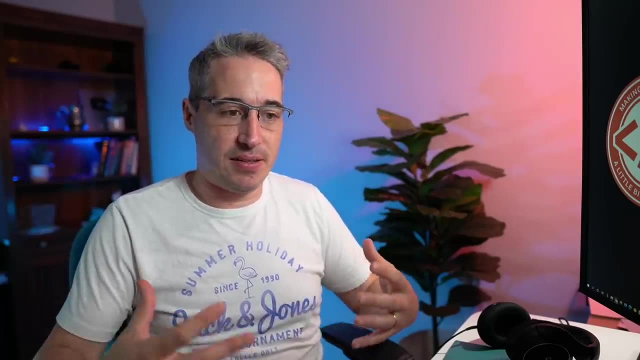 two sites for one site was stupid, so luckily that didn't really become a thing, but we did have to evolve our mindset on how to make layouts and I think the most important thing, the thing that I've said that has hit home the most for most people when it comes to mindset- is that one thing you? 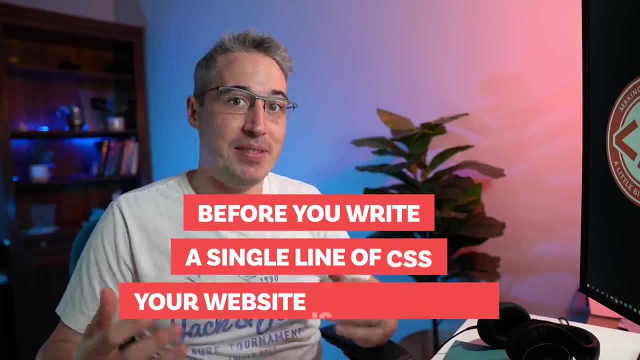 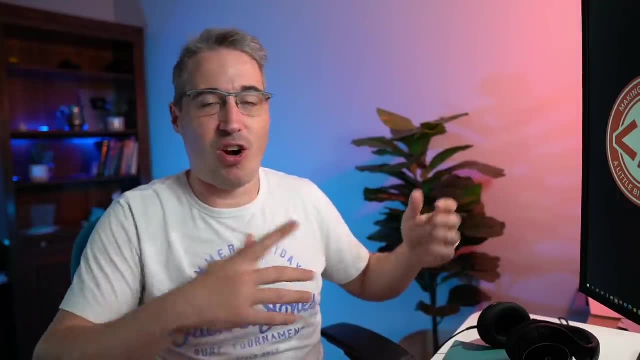 have to remember is before you write a single line of CSS. your website is responsive. the layout is going to work on really big screens and really small screens might not be pretty. on really big screens it might be kind of hard to read, even because the line lengths can get really long. but 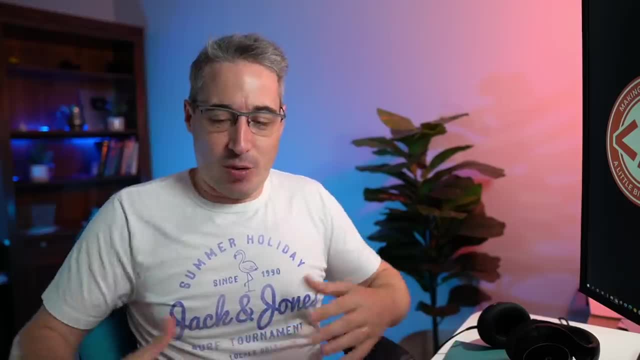 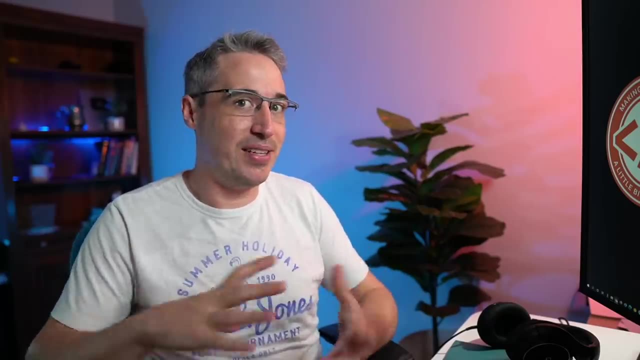 the website adapts to the viewport. So that's the first tip, No matter what you do with it. I know images can overflow and that sort of sucks, but we're not losing our text, we're not losing anything along the way and I think understanding that in embracing that that can 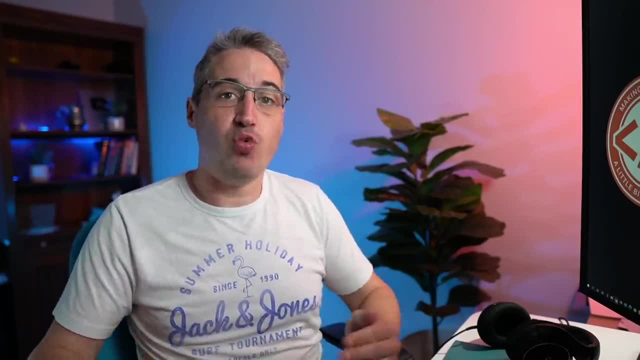 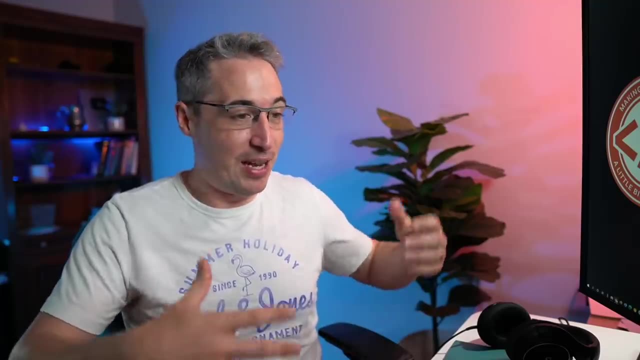 really help us out. when we're writing our CSS- and it's also when you do run into issues- the thing to consider is: you're the one who wrote the CSS that's causing that issue. because you wrote some CSS. it was working at one screen size, but it broke on other sizes. it's that CSS that you wrote and very often, 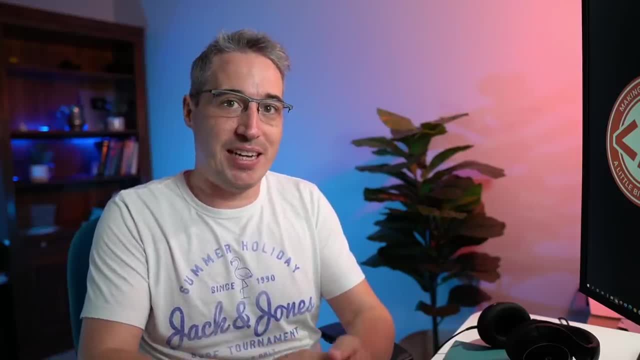 from my experience, that means we actually have to take a little bit of a different approach in getting things working, And that's what we're doing. That's what I want to look at with you through the rest of the tips that I have for you today. 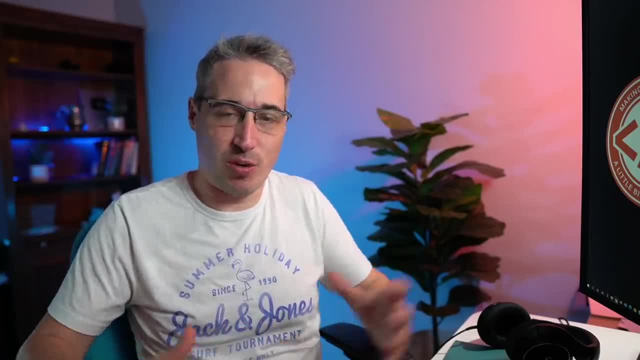 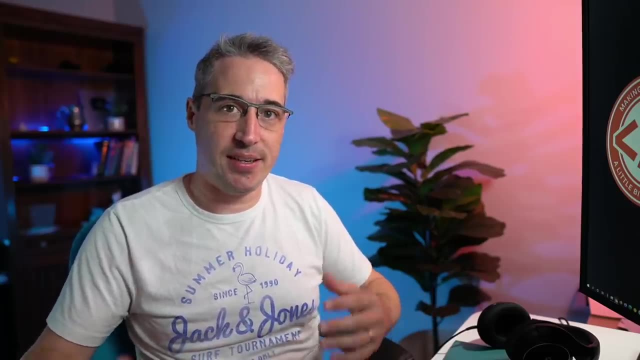 So, because it's us who are causing the problems, my first suggestion to you- and we're keeping this together with mindset and it's embracing this natural responsiveness of everything- is, when you start writing your CSS, start first, global first, like the things that kill the most, birds with one. 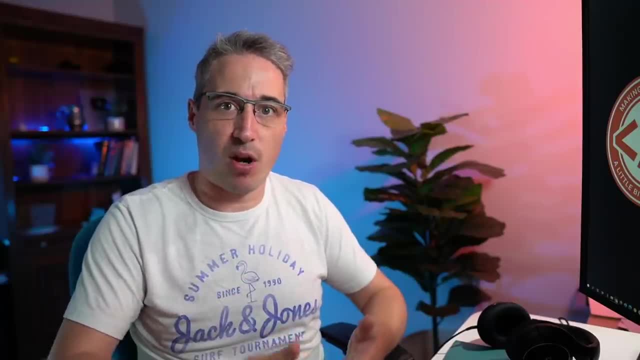 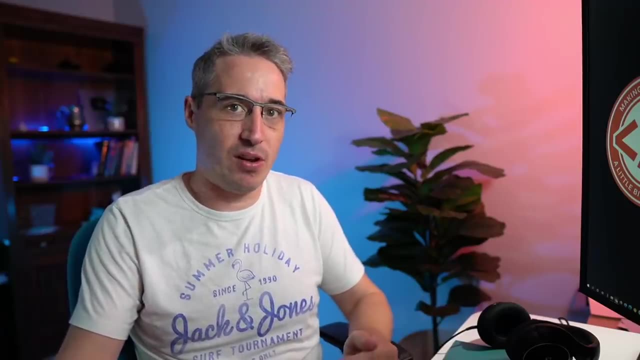 stone, but don't worry about your layout. first cover things like typography and colors and sending backgrounds and all of that. it's actually going to get your site pretty far along the way without having to even worry about your layouts at all, with the really big added bonus that your mobile 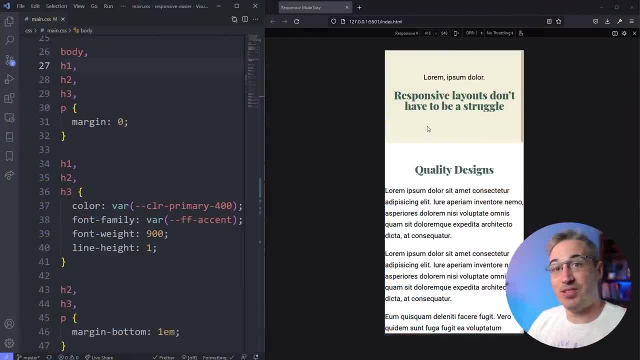 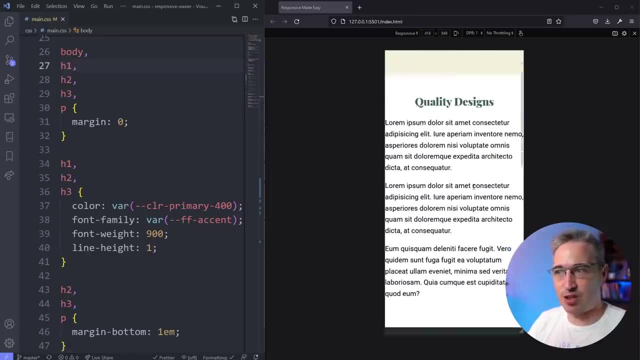 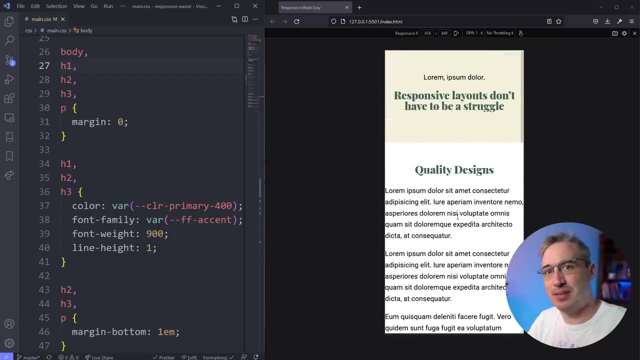 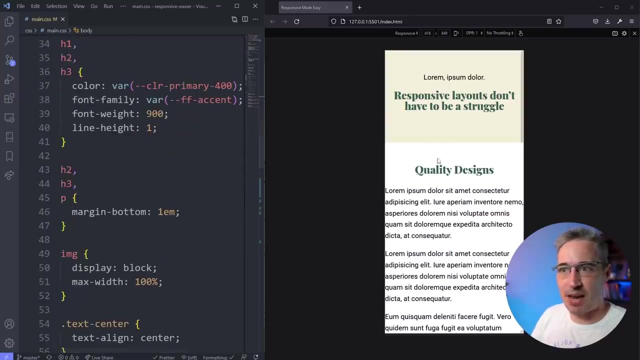 layout will be finished, but it's not going to be terrible by any means. So here's an example of a site where I've started doing things and I've stuck as simple as possible and you can see like there's issues touching the sides of the screen and a few other things, and you know there's some spacing issues, but overall it's working. everything is stacking and it's a very simple site. but you can imagine on more complicated sites as well, as you do things and all I've done here is my colors, I've set backgrounds and I've put a little bit of padding for each one of these sections. 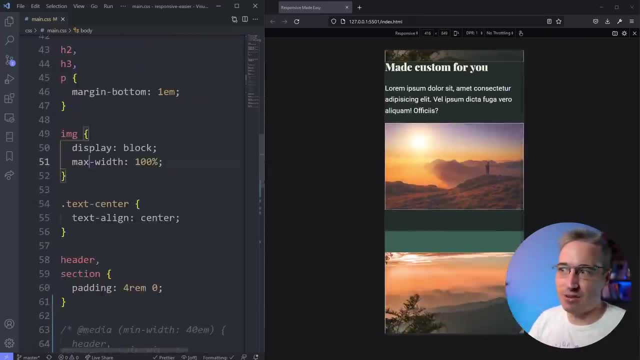 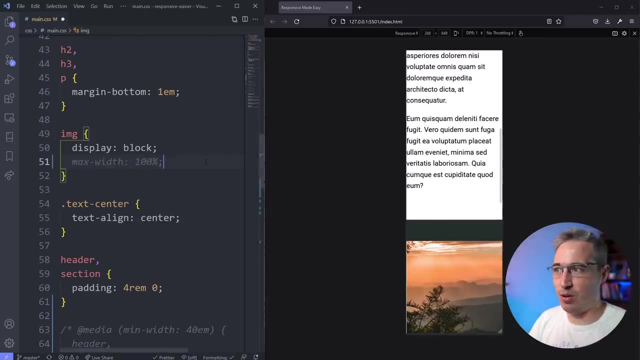 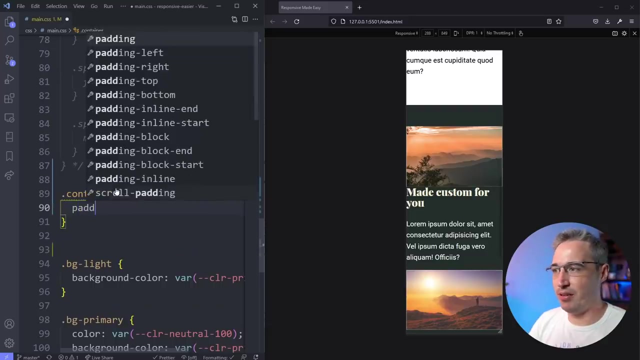 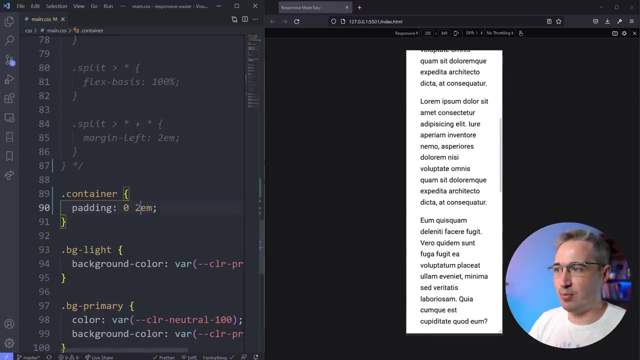 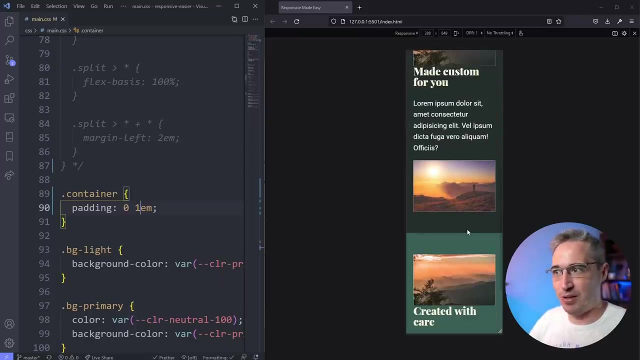 That's it. There's nothing too fancy going on here At all, and I've also done this on my image. just again. we don't want our images to be overflowing, which can happen, so this is a nice, simple one right there. a max width on your images so they can adapt to their container. so then I can come in and I have a container in my HTML already. but I could just come in here and say padding zero on the left and the right and two M on the right and the left, and then I even- maybe that's a little big, actually it's good with one, and I've solved that problem of my text touching the side, so it doesn't take a lot for the mobile layout to be responsive. 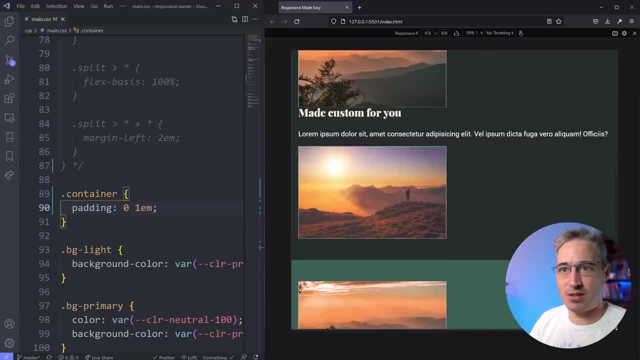 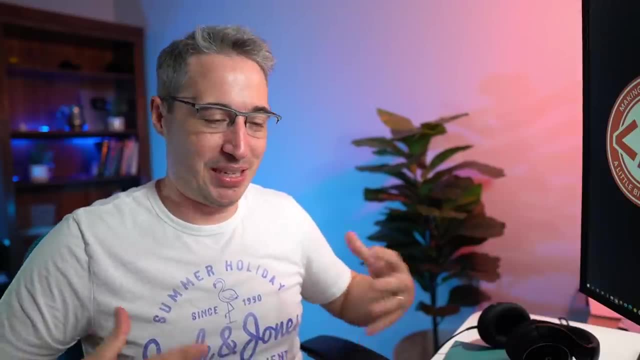 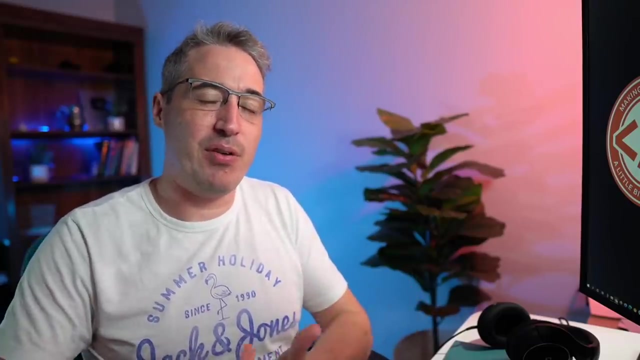 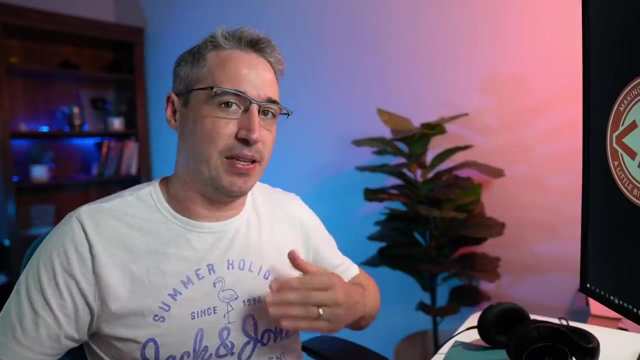 And, as I said, the layout will be responsive. as I grow this, things are going to grow just fine. it doesn't look pretty, but it's not broken. somebody could access this site and it's going to be perfectly fine. now you're saying: but Kevin, I don't want this ugly layout like that, I want something that's a little bit more, and I totally get it. so the next thing is, when you start thinking more about layout, the very, very first thing I'm going to suggest is avoid fixed sizes. when I say fixed sizes, I mean things like width, 1000 pixels, height, 500 pixels or whatever it is setting like a fixed height or a fixed width. it's only going to be a little bit more responsive. 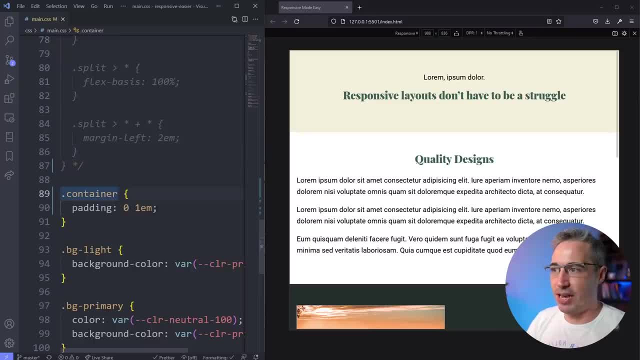 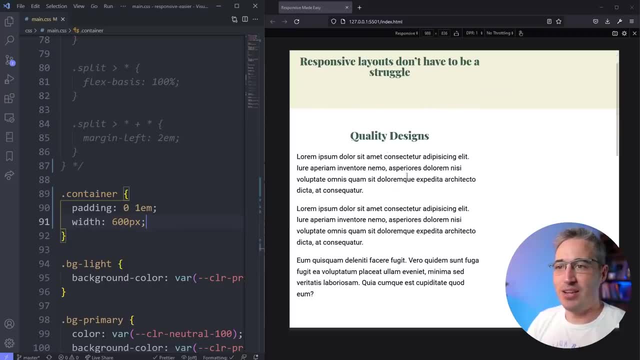 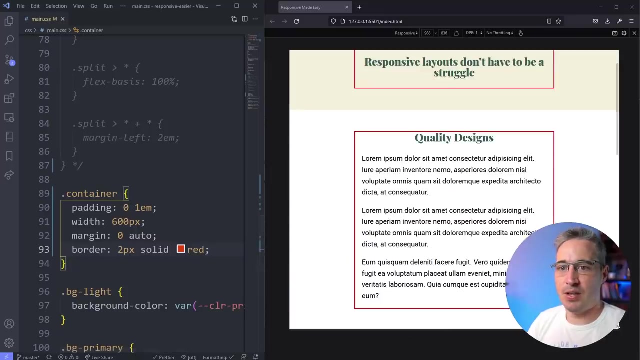 Cause you problems. so if we jump back into the editor here where I had my container, if I come on this and I give this a width- let's just say 600, so I think that will fit within my viewport. there we go. so I get this locking in at 600 pixels and we can even do the margin zero auto to center my containers on the screen and let's give them a border as well. just, we can visualize a bit more: two pixels solid red to make it easy to see. so you can see I have a container and all those spots and it's doing its job, it's holding the content in the center. but when I 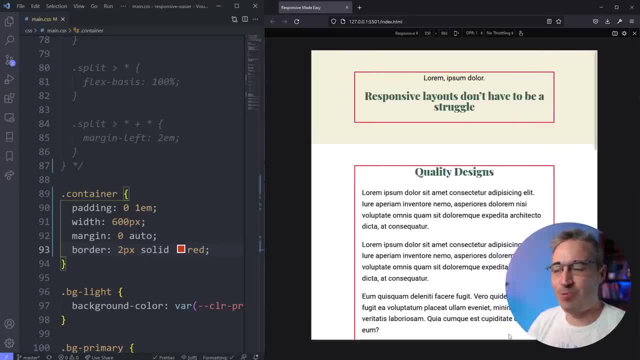 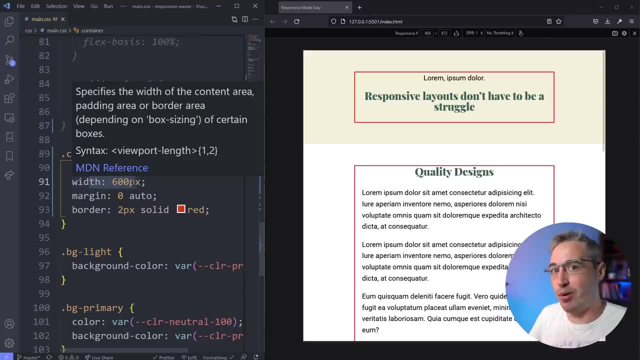 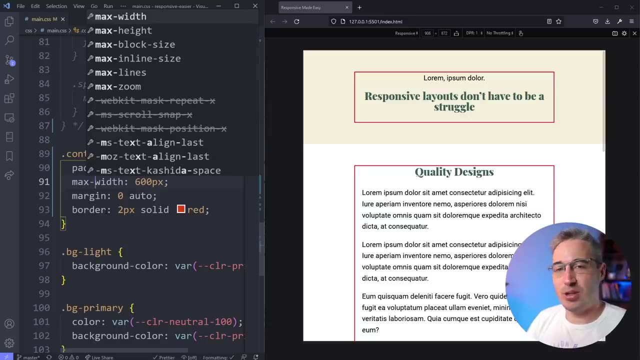 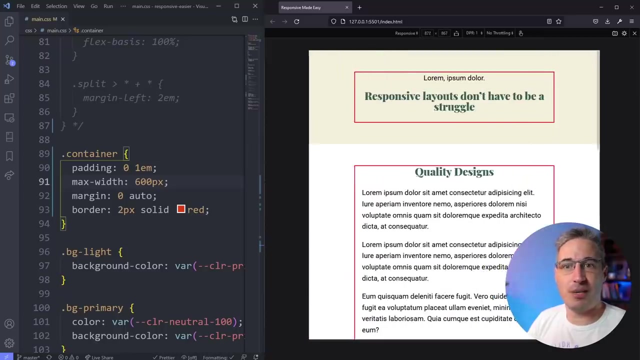 go smaller than that, it overflows, and that's terrible. one thing I see people doing with something like this is they actually come through and they start doing a width and then they make a new media query to change it and then another media query to change it. we're going to talk about media queries in a minute, but here instead of that, I could just come on this and say max width, and so I don't have a set size, but I have a maximum size. so now, as that gets smaller, it will be allowed to shrink, but if I get too big, then things can go that way and I think 600 is a little bit small. I personally work with ems and rems most of the time. 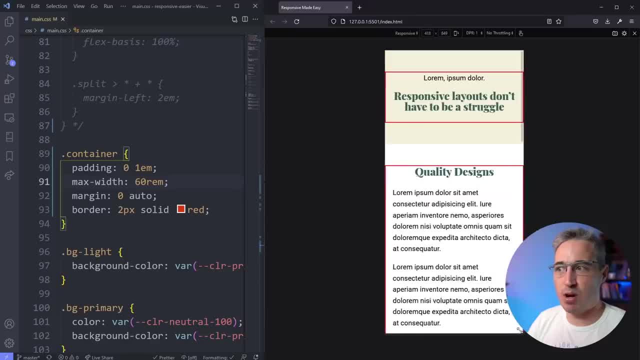 of the time. So I'm just going to throw in a 60 rem here. There you go. I can shrink smaller than 60 rem, but I can't get bigger than that size. And you can see that it's working everywhere and 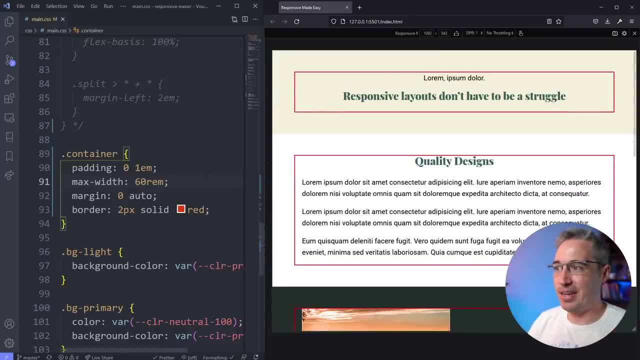 it's perfectly fine. So I don't have any overflows, and that's awesome. And an even bigger issue, I find, than widths, because people have an easier time with this But say we go into my header and I say a height, and heights are like the bane of my existence. Don't set fixed heights, is my. 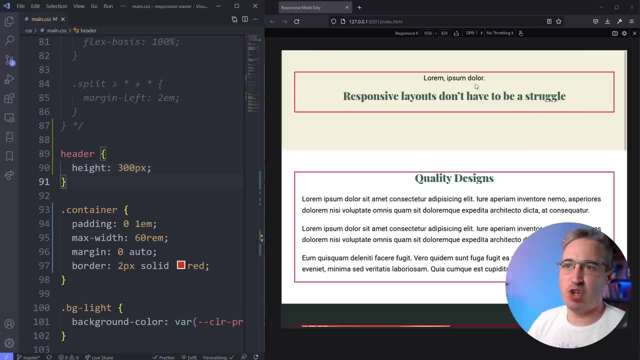 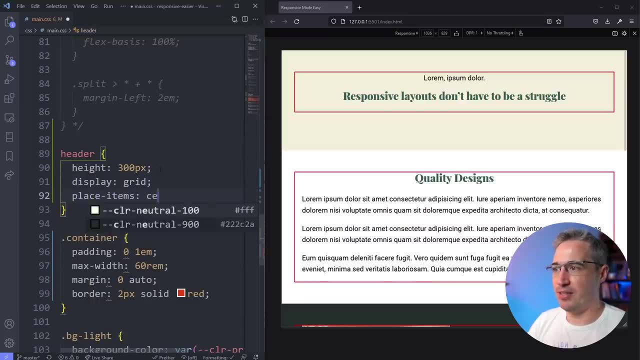 general rule of thumb. So there you go. You can see I set it at 300 pixels and you know, use flex box or something on there, so we can even do that display. I'll do a grid, because it's easier, And then a place items center and it centers that red box perfectly in the middle and you're super. 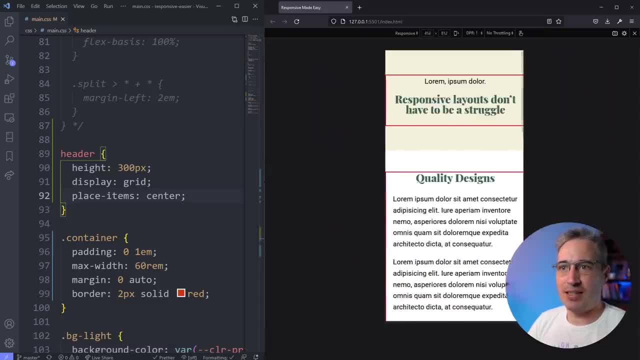 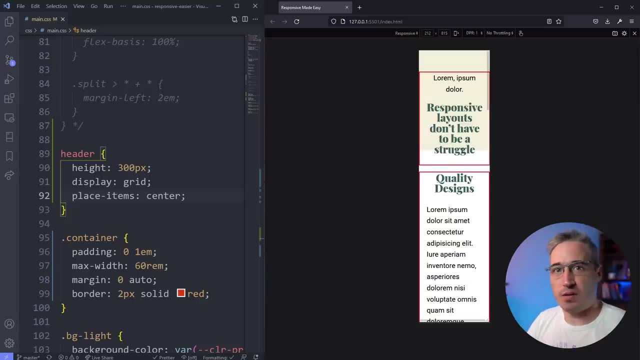 happy with yourself. But then you run into this issue where, as the content gets longer and longer and longer- and I'm exaggerating, but I don't have a lot of content- This spills out the bottom and it overflows, And that's because I've set a specific height on that. We can exaggerate it. 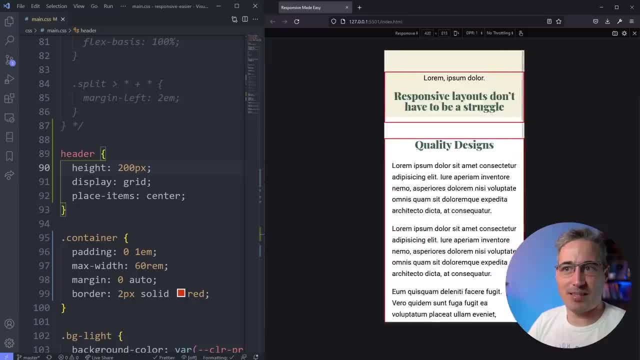 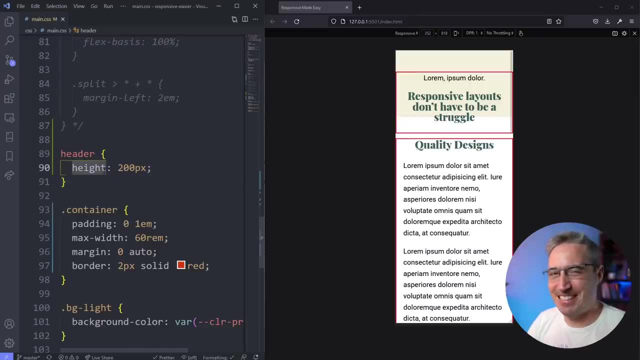 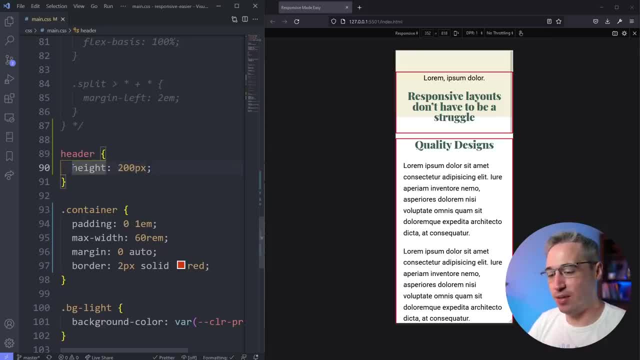 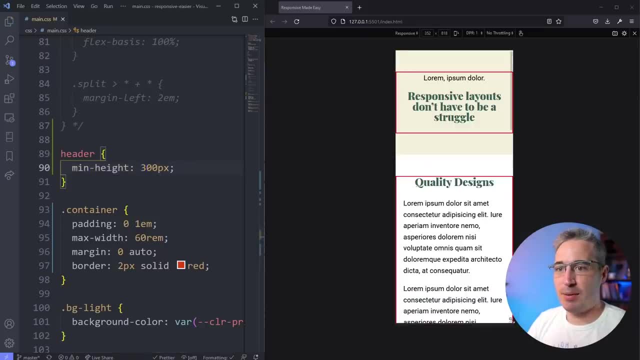 dangerous property to be setting. But there is a solution. Again, don't use fixed ones, but you can use ones that can adapt, So you can see a minimum height And so I could say it's a minimum height of 300.. And that means over here, you'll see, actually like it's not balanced out. 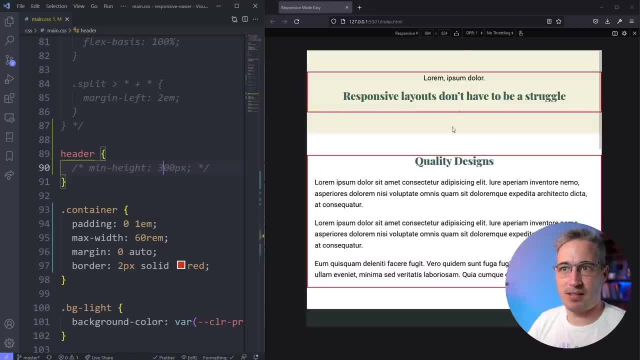 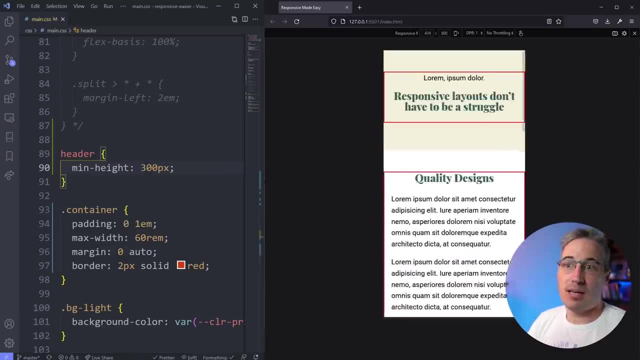 If I take this off, we can see it will get smaller And this is my padding that's giving me that space. So what I can say is 300, it's gotten bigger, So it has to be 300 pixels or, if it runs into a situation where the content is getting longer, that it's going to. 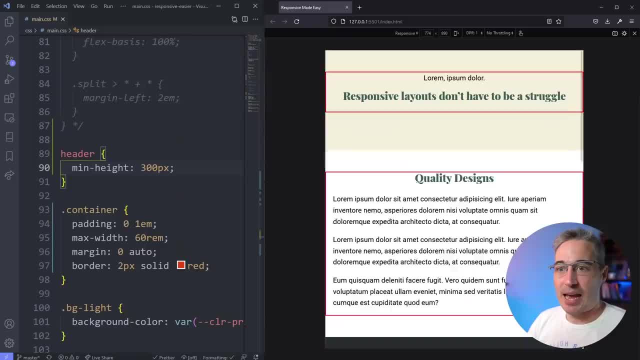 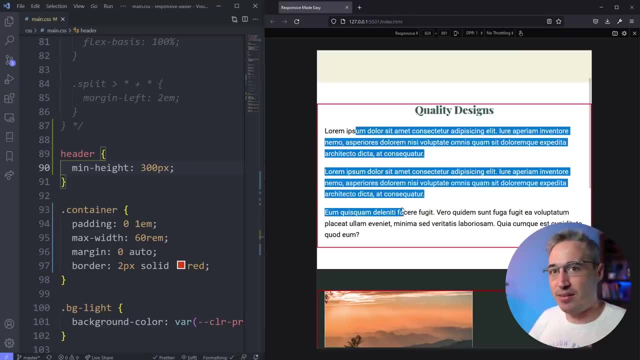 it will grow to adapt to that, just the way it naturally would anyway. And it's, it's a basic thing of area, right? This text here- and we'll just move down to here- This text here has a certain area that it needs to live in. So width times, height, as viewports get narrower, that 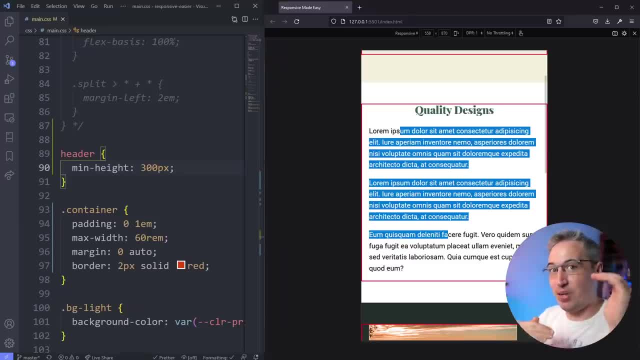 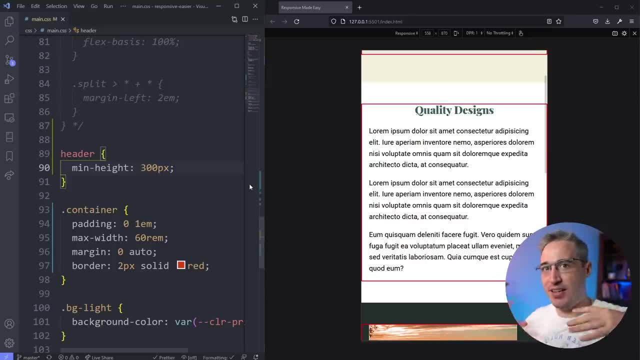 means that that this is shrinking. So to keep the same area, we need to grow the height. And if we set fixed heights on things, that cannot happen. So even if you're setting a like 100 viewport height, because you have this big hero area that needs to fill up the whole, 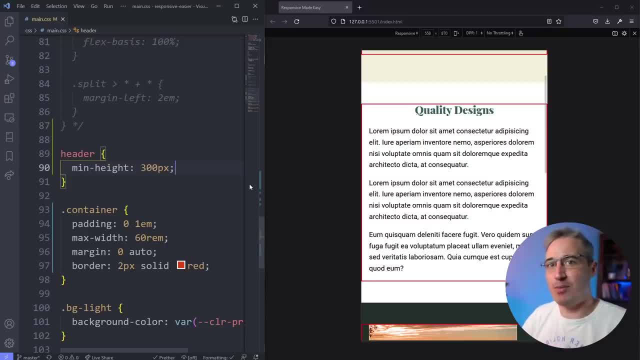 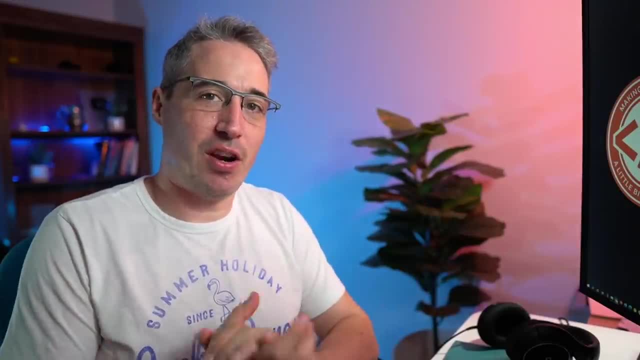 thing. setting it as a min height will just solve potential problems that you could run into when you start going on to narrower viewports. Now I promised we would talk about media queries, and media queries are something that I think are still an important part of web development, And a few of 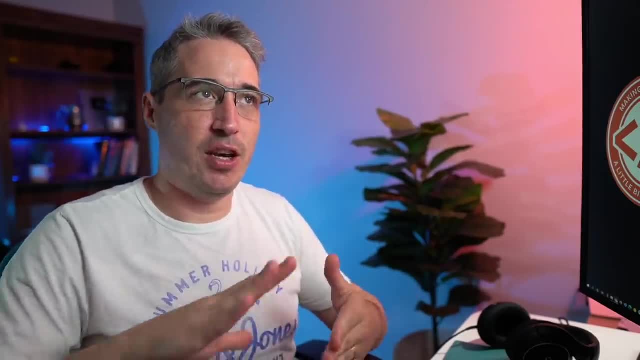 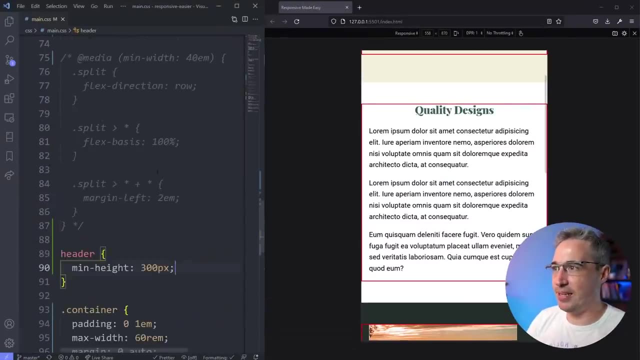 my points here are actually going to talk about them, But the first thing I want to say is: try as much as possible to use your media queries to add complexity. So what I mean by that is, if we come in, I have this split class that's here, which is what I'm using to create my columns, And I'm just 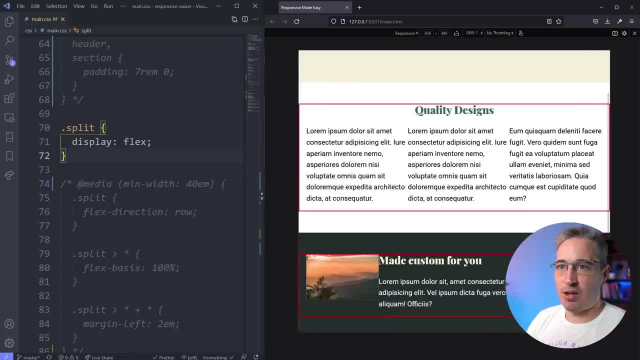 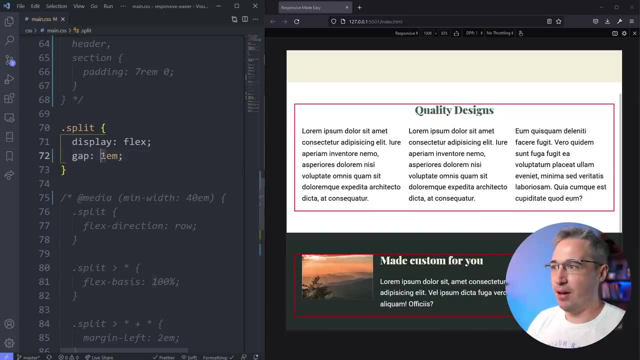 going to take this off first, So you can see here that's come in and created columns And I want that at my large screen sizes, And so then I also come in and we have flexbox gaps now, which are the best, So we can do a gap on that just to space things out a little bit more, And you can see that. 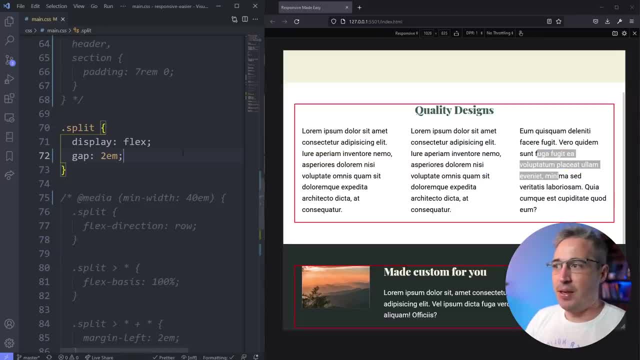 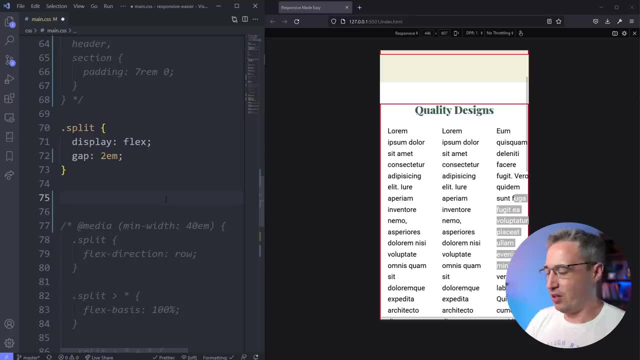 it's coming through and it's working And I'm getting my three columns here, which is awesome. But then when I go to small screen sizes, well, that's kind of annoying, right Like we're shrinking down, it's getting too narrow. So then you come in with your media query and you're like: 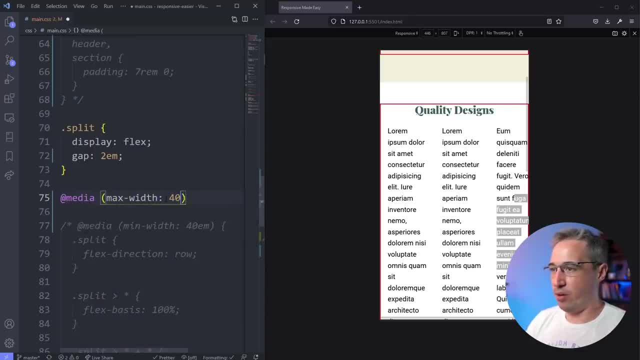 okay, I'm going to go in with your media query, So app media, and you do a max width of 40m, And we'll talk about why I chose 40m after as well, And then we do our split And in here, then you. 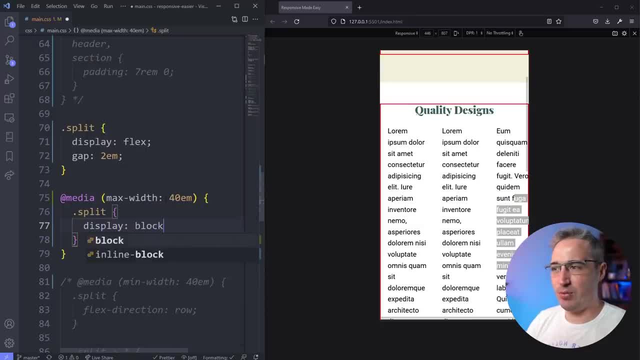 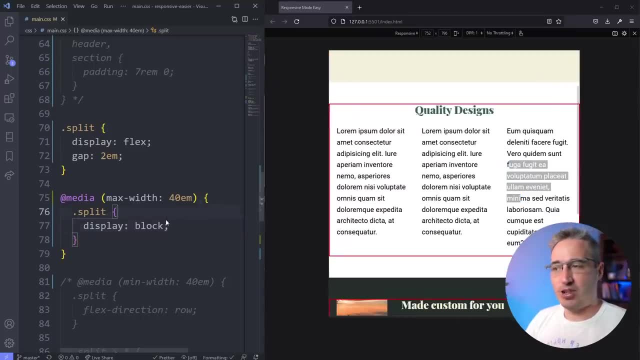 say that the display is, I guess you go back to block, which is the default, or you go to initial, which is a little different actually, But you know, then I get this thing going on, But what I'm actually doing is overwriting the default that we had here in the first place. So what I could do. 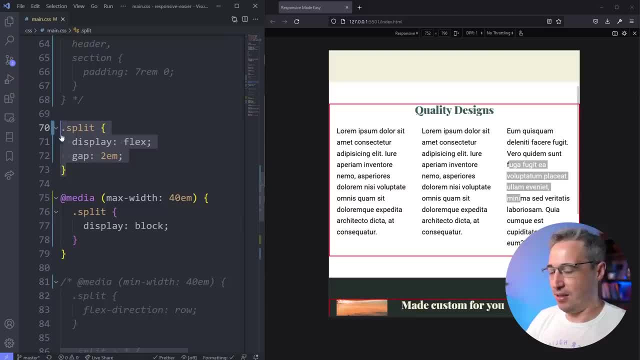 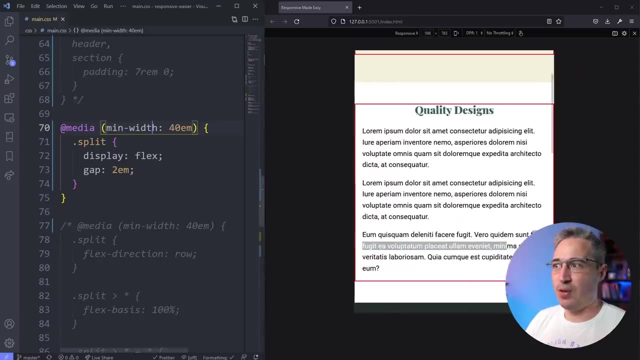 if I wanted to is I could actually take this and put it in my media query And delete this completely and switch this over to a min width, And that's going to give me the exact same result And this is a really simple solution where I'm. 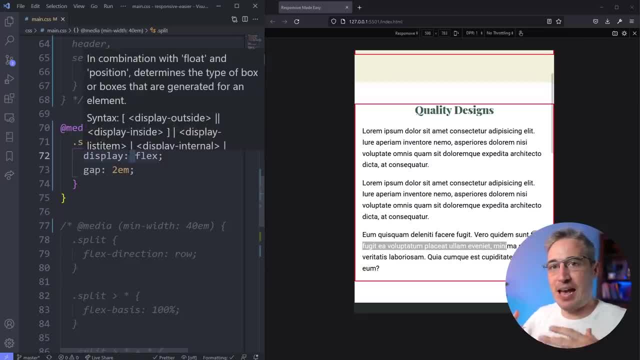 only doing like a display flex. But what I'm doing is I'm instead of adding- instead of adding the complexity in and then having to overwrite a whole bunch of properties that I did in the first place- what I'm doing is just adding that complexity when I need it And in general, desktop designs happen. 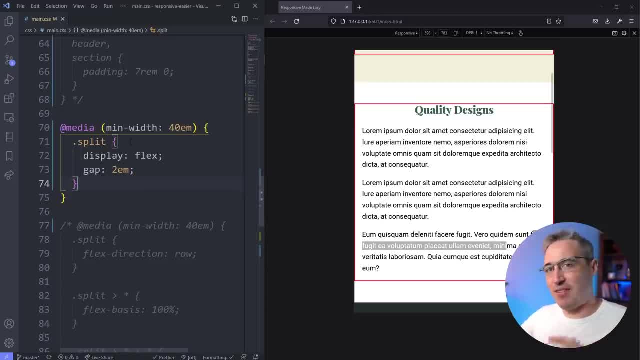 where things get more complicated, The bigger the screen. you get columns, you get fancy things going on and all of that stuff. So in general, and like 99% of the media, queries I write are min width ones. I'm doing mobile first. And again, when I say mobile first I just mean I'm doing all. 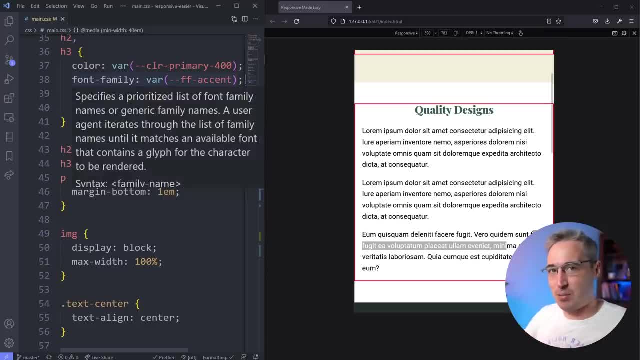 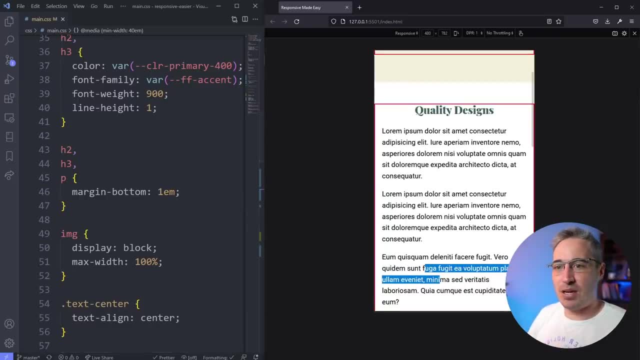 the things I talked about in the previous tip: Doing my colors, my backgrounds and then a bit of spacing. And then I'm going to look at it and go, okay, that looks pretty good on mobile- Maybe I have a few tweaks to do- And then I go, okay, now I need some columns. So where are those columns? 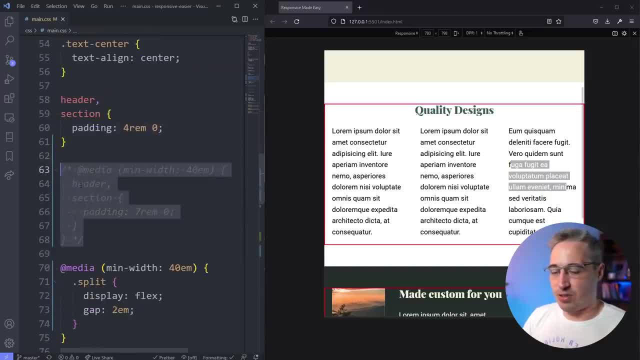 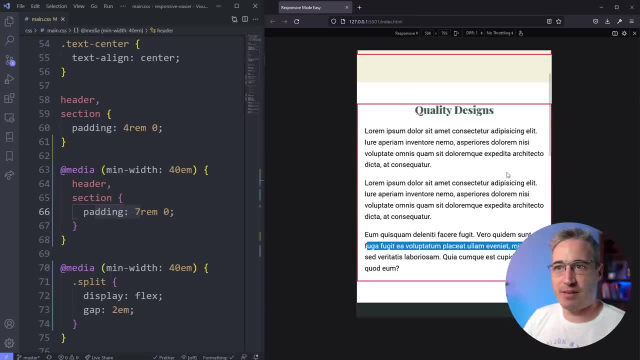 of complexity in. Now I have one that's commented out here. So, just as another example of something you might need to do, something like this where you are overwriting a property to change it, And that's perfectly fine, And that's where I have less padding when I have a narrower viewport. 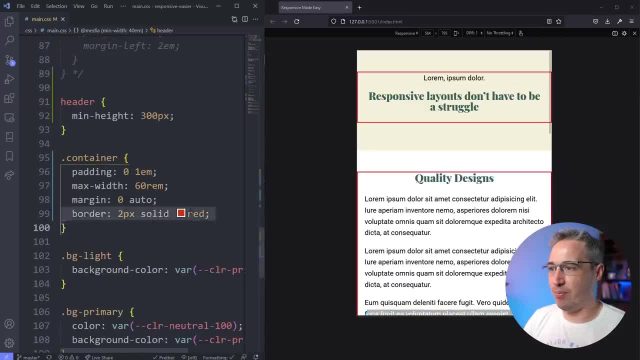 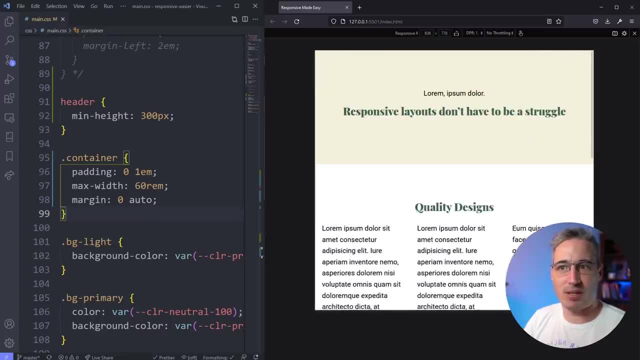 And let's turn off that red container because it's driving me nuts. But we have less padding because we don't have as much screen real estate And then that padding increases at larger screen sizes. So personally like something like that: yes, you're going to have to overwrite some things. 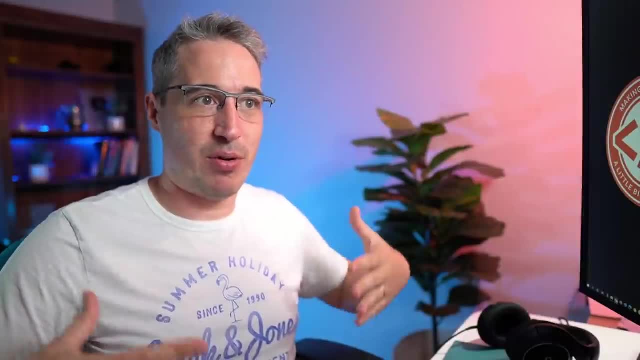 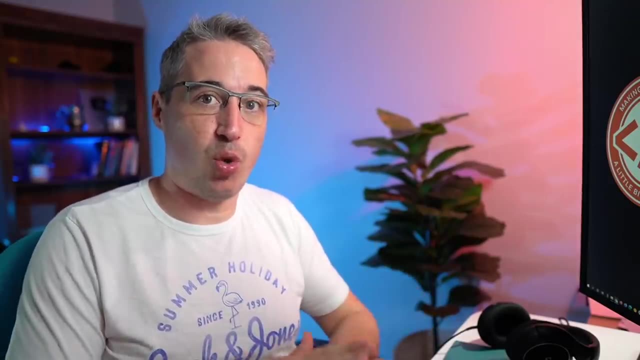 that's completely normal within a media query, All right. So I was talking about having breakpoints before and how I was going to, how I chose 40M And really for me, it's about where the layouts start to break when I'm creating one. So if my layout when those columns are just getting too, 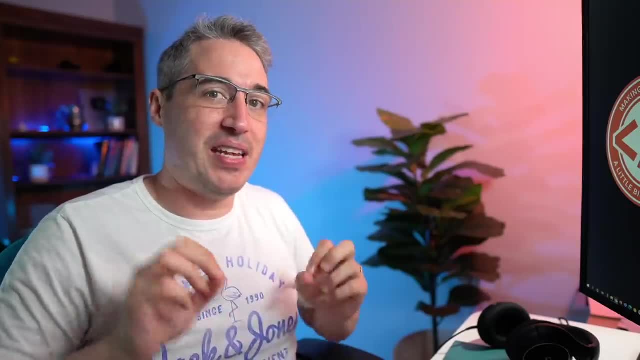 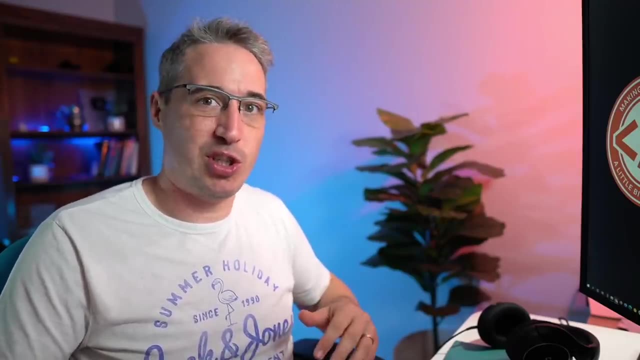 narrow. okay, I need a breakpoint there to stop those from getting too narrow. But the other thing that's really important is I try to avoid having too many breakpoints And I find for a lot of designs you can get away with one, sometimes two breakpoints, And sometimes you need something very 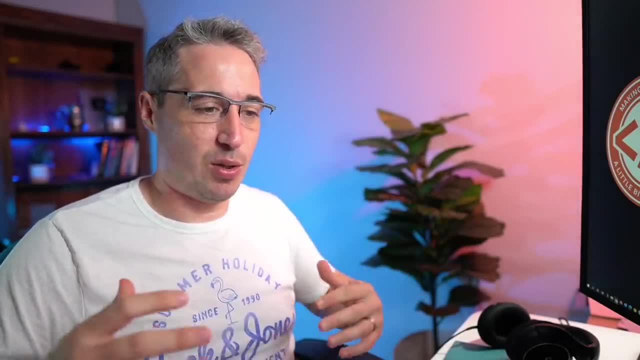 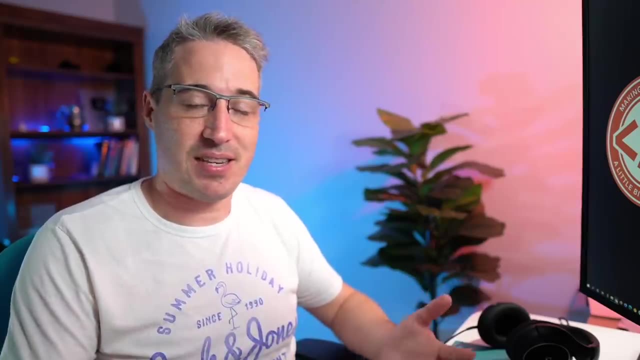 specific for one thing, But a lot of the time you're going to have a lot of breakpoints that you can do general groupings. So all of my breakpoints happen to be happening at 40M And it just so happens that's where, in that layout, based on the font sizes I have, and all 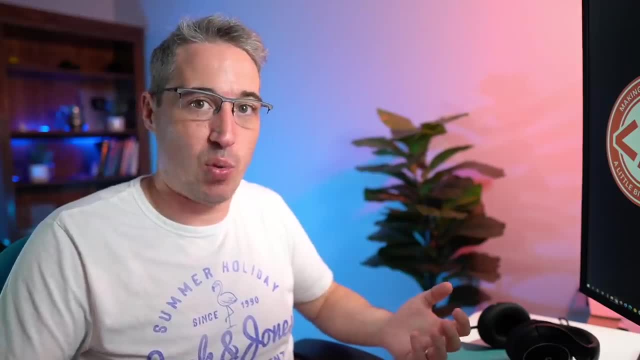 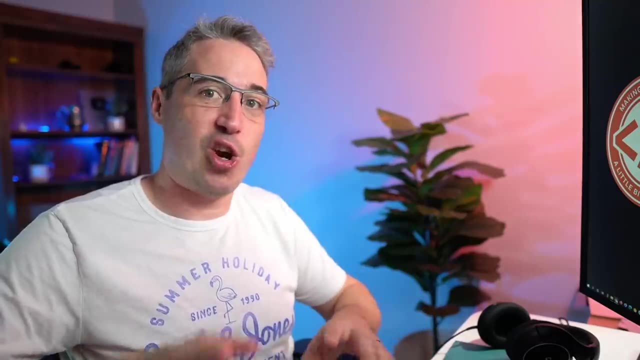 those other things. that's where the layout worked And that's where that breakpoint worked really well, And I just make general observations on that. with the design Now, another thing that I realize is you might be writing code and not be a designer and you're not too sure or comfortable making. 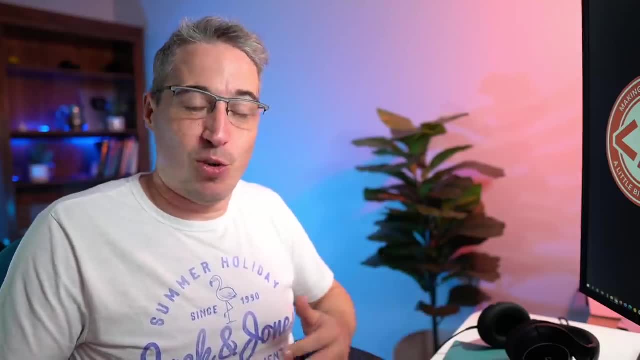 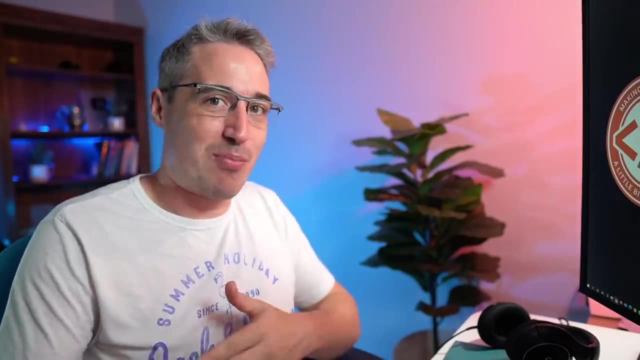 those decisions. If you're writing CSS, that does come down to you. But if you do have a designer you can talk with, then talk with the designer. And if you're writing CSS, then talk with the designer and see where he thinks things should be changing at. But you can always round up round. 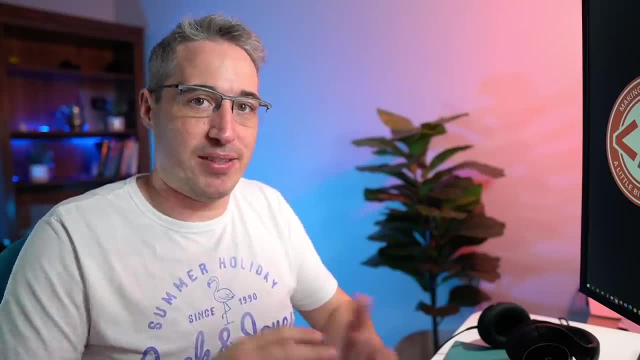 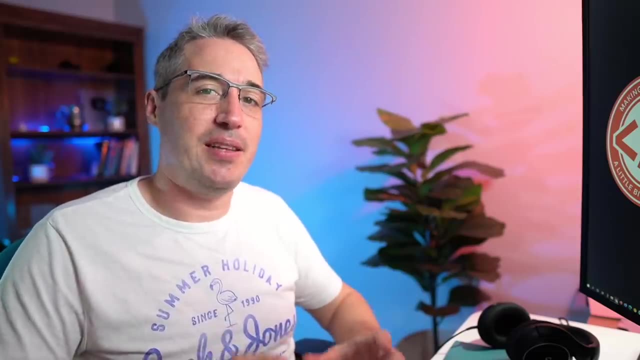 down to try and get everything happening within the same breakpoints, instead of having 18 different breakpoints to try and maintain, which just would be a complete nightmare. And also on that note, I would completely avoid doing device specific breakpoints. We have way too many devices now. 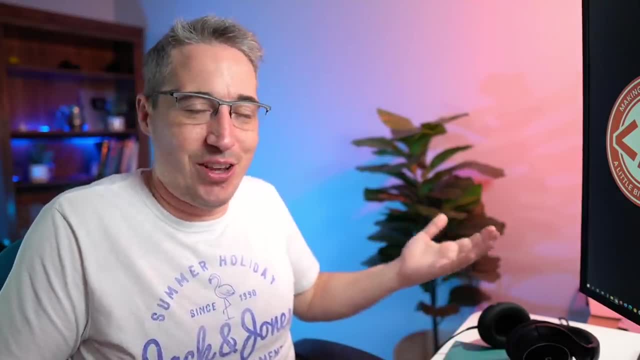 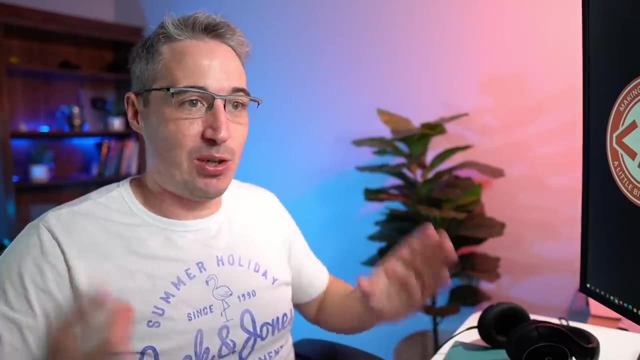 even like an iPhone. like which iPhone are you going to target? And there's so many different of every single device that's available right now And every single screen size is available. So just look at your layout and see where problems are occurring and adjust it from there and make 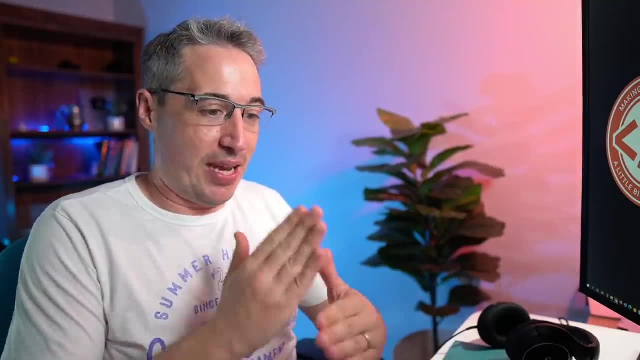 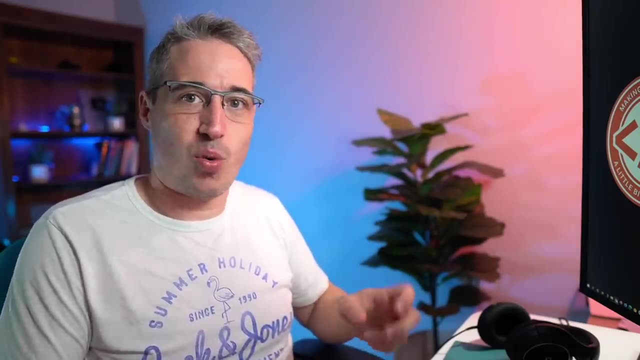 those tweaks that you need to make instead of worrying about. okay, at this screen size, then this one, then this one, or on this phone it looks like this, because then your buddy next to you is going to have a phone that's 15 pixels wider or 20 pixels narrower, or 20 pixels taller or whatever. 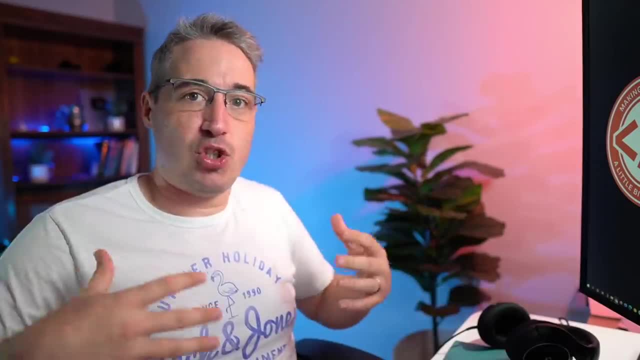 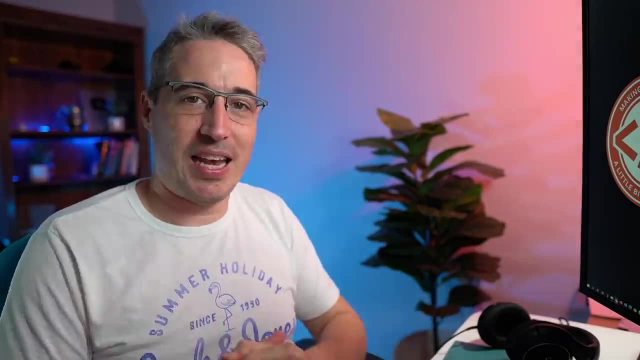 it is Like the differences between them. it's just there's too many variables there. And if you start going device specific, it's just you end up with too many devices that you'll have to worry about. And tip number five is to use more modern CSS approaches So you can get away. 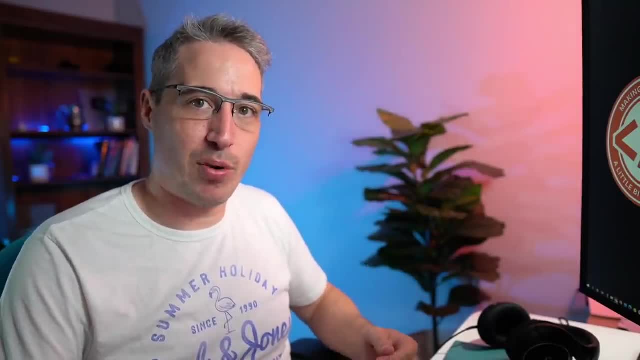 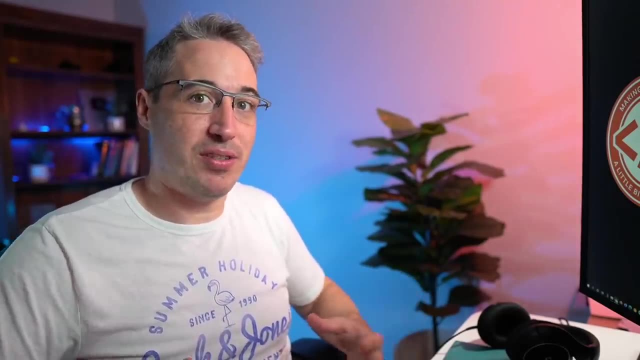 without even having to make these decisions. Sometimes you don't have to worry about break points as much. A lot of people rally against the idea of even having break points in the first place, And with modern CSS we can start moving away from them. I don't think they're the devil. 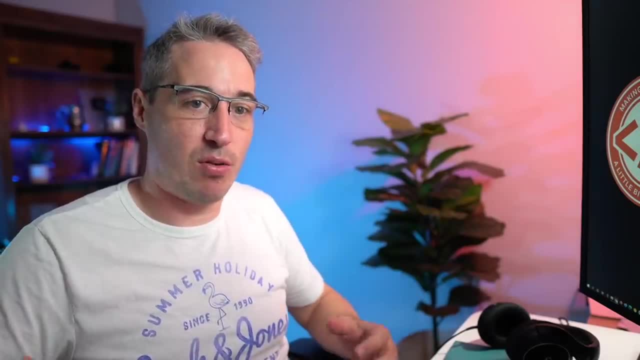 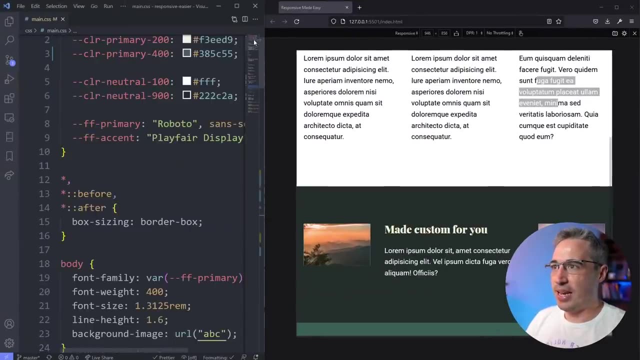 I don't think we need to get rid of them, but we can start moving away from them and going more based on intrinsic design and stuff like that. So if we jump back into the browser here, one way actually- and I don't necessarily like this, with small font sizes but with really large ones- I 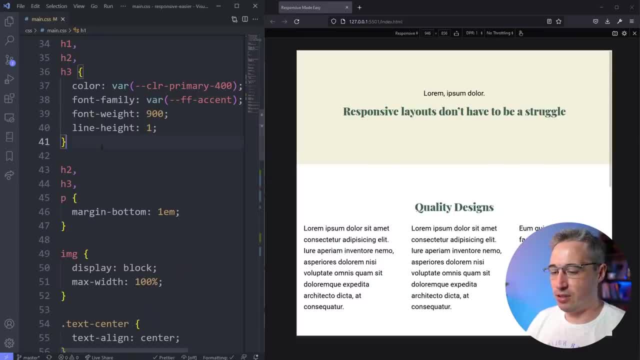 think it's a decent way to work. So here my title that I have. what I could do is come in and select it and say that the font size is a clamp And this is going to clamp it between a minimum and a maximum font size. So the smallest I want it to go to is three rem. The biggest I want it to go to 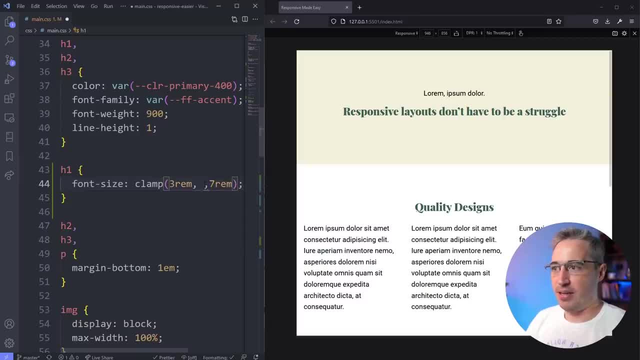 is seven rem. And then in the middle of that I can come in and say that this should be a one rem on another line, just so it's not going off screen. So we can do a one rem plus, say, 10 viewport width. There you go. It just got gigantic, but you'll see that it will actually shrink with my. 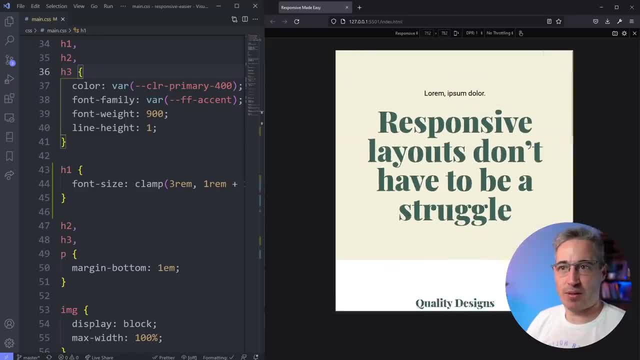 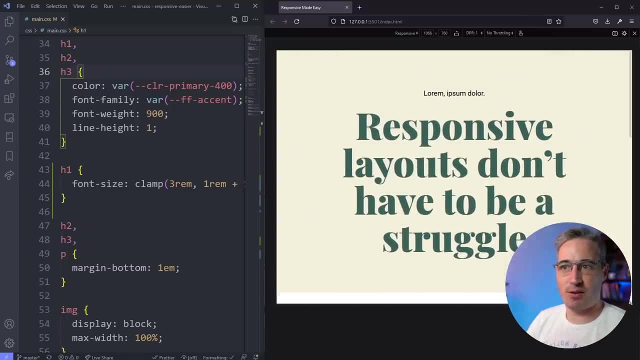 screen, or grow with my screen or viewport size, the viewport width here, and it will hit a maximum size at one point. So here it's not actually getting any bigger or smaller, even though I'm changing the size of the viewport. And then here it shrinks, shrinks, shrinks, but it will hit a 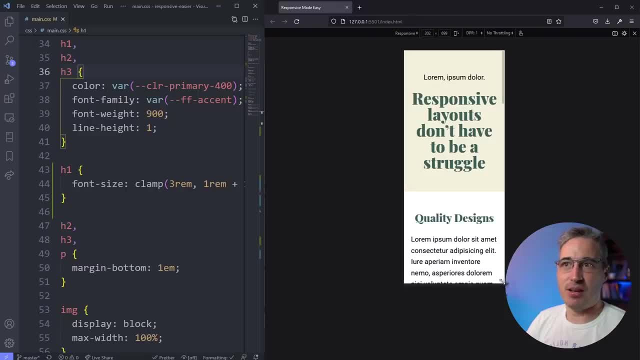 minimum size at one point and it will stop shrinking And I can see that's actually. we're down to 300. So I don't even have to really worry about but again you could come in and say this should actually be a two instead of a three. 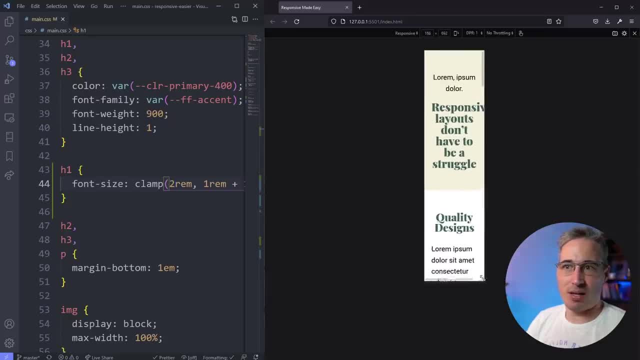 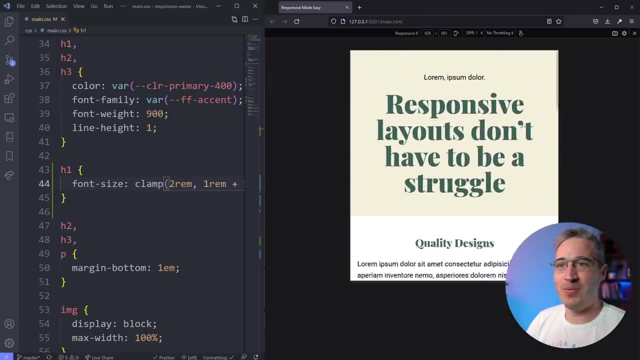 And then that could actually continue to shrink down. at one point They will lock in and stop, though, And again, don't worry about like 270 width. Nobody has a phone that's 270 width, So unless you're trying to do it for a watch maybe, but you know 320, if you really want to. 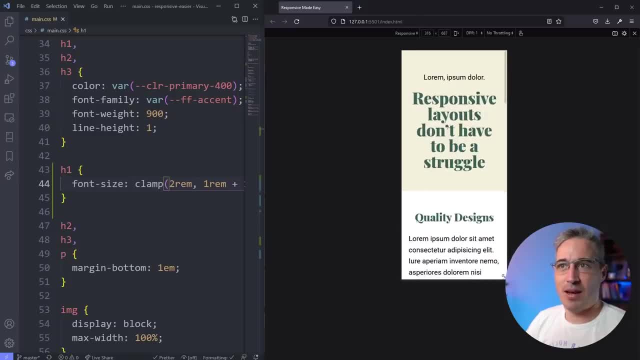 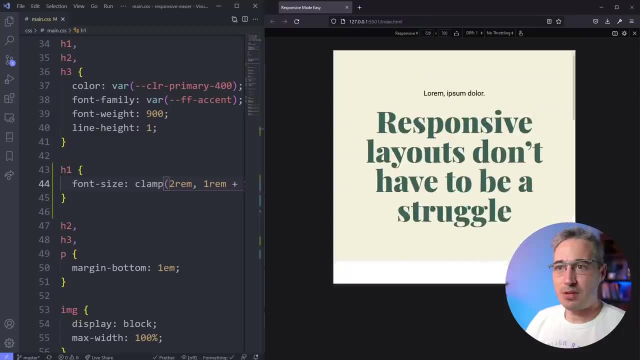 be careful, and a lot of modern devices are at 370, I think. now I usually do 320 just to be on the safe side. though It's like the iPhone SE and the SE2, I think we're both in that range of 320. So yeah, 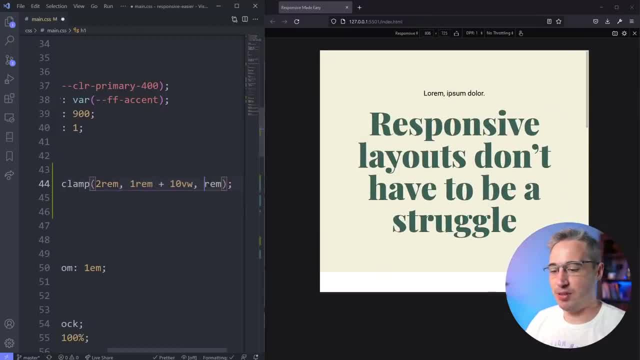 that's a nice modern approach And actually I'm going to clamp this just a little bit smaller, just so we can really see how it's working. So you can see it's shrinking and then it clamps there and it stops growing And you can.